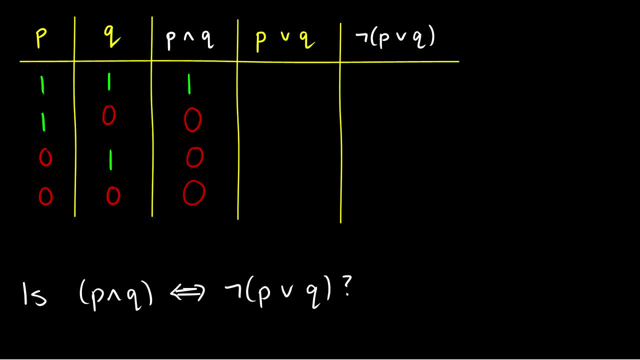 this is 1, 0, 0, 0.. Now for P and Q to be logically equivalent to not P or Q, then this would also have to be 1, 0, 0, 0. So let's see if that's the case. Well, P or Q, What are the truth? 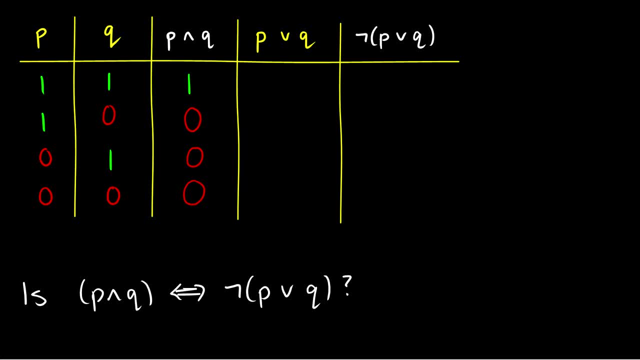 conditions for P or Q. Well, P or Q is true when at least one of P or Q is true. So it's going to be true in the first three rows, because P is true in the first two rows and Q is true in the. 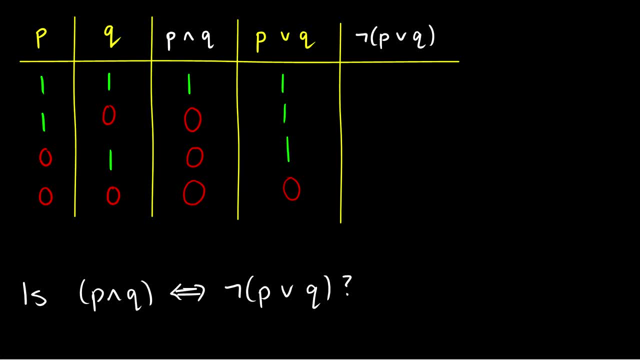 the third row, but it's going to be false in the fourth row because p and q are both false. Now, not p or q, we just take the negation of the previous column. So 1110 is going to become 0, 0,. 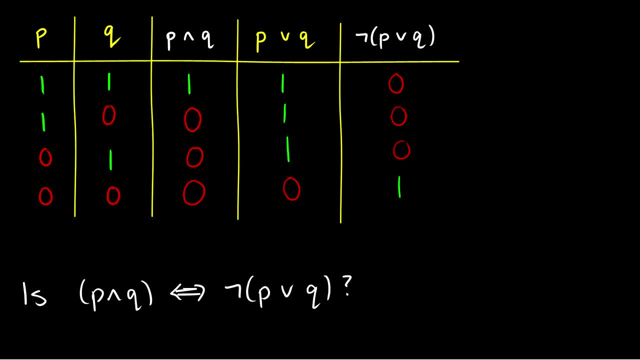 0, and 1.. And of course I'm just taking the negation of the previous column. So are p and q, and not p or q, logically equivalent? Well, the answer is no. And why is it? no, It is not equivalent because the truth conditions for p and q and the truth conditions 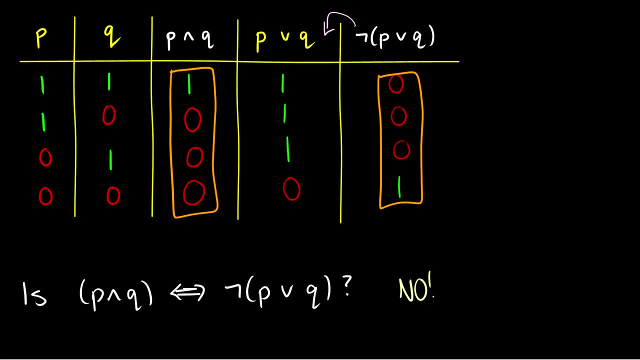 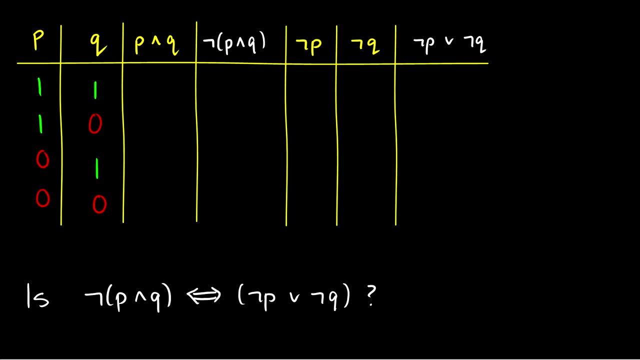 for not p or q are not identical. Therefore these are not logically equivalent. Let's do another example. Let's ask: is not p and q logically equivalent, p and q logically equivalent to not p or not q? So we just did p and q before. So first, 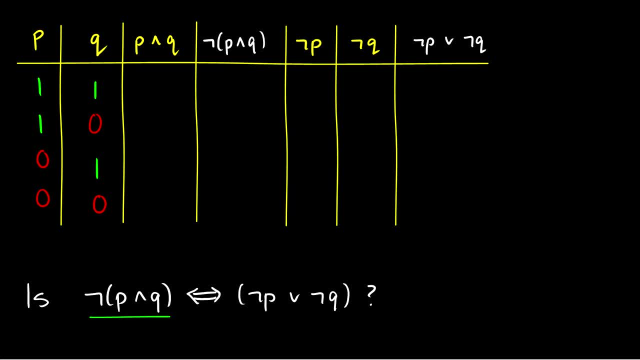 I'm going to do not p and q, So I have to build p and q before I can build not p and q. So p and q, we just did this. This is going to be 1, 0, 0, 0.. Now, if we take the negation of that, 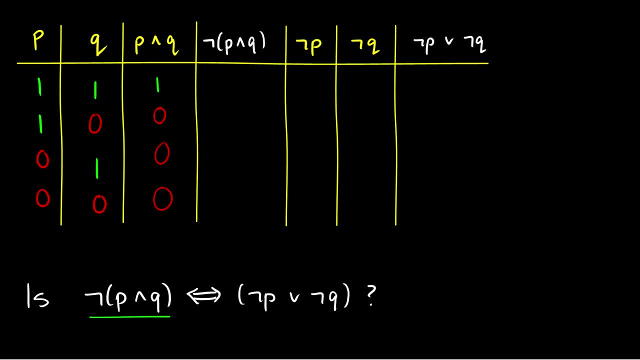 the values just flip, So not p and q is going to be 0, 1,, 1, 1.. Okay, So we have the truth conditions for not p and q. Now we have to do not p or not q, But in. 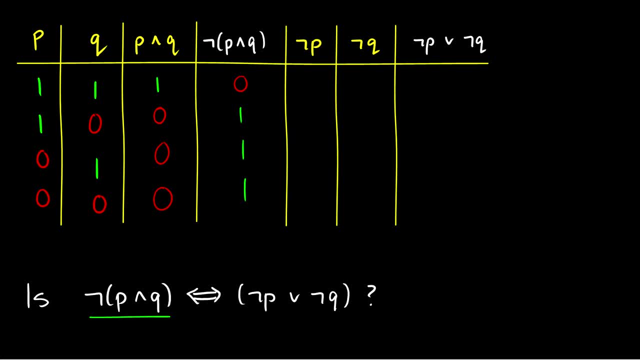 order to do not p or not q. first we need to do not p, then we need to do not q, and then we can put them together with: or So not p. This is just the opposite values of p, So if p is 1,. 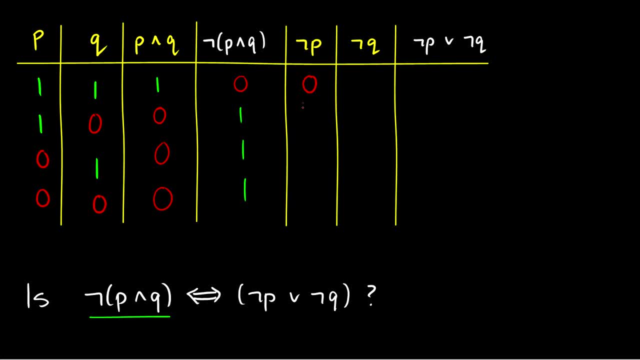 1, 0, 0, then not p is going to be 0, 0,, 1, 1.. And again, just to connect these visually, this p column changing to not p, we just reverse the values. Similarly, with the q and not q column, we just reverse the values again. So instead of 1,, 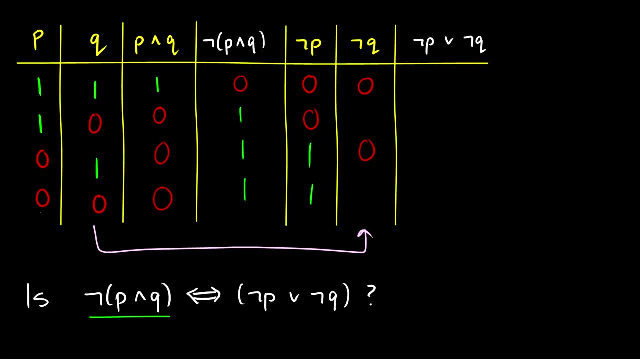 0, 1, 0, it's going to be 0, 1, 0, 1.. Okay, So now that we have not p, not q, we can do. not p or not q. So not p or not q is going to be 0, 1, 0, 1.. So now that we have not p or not q, we can do. 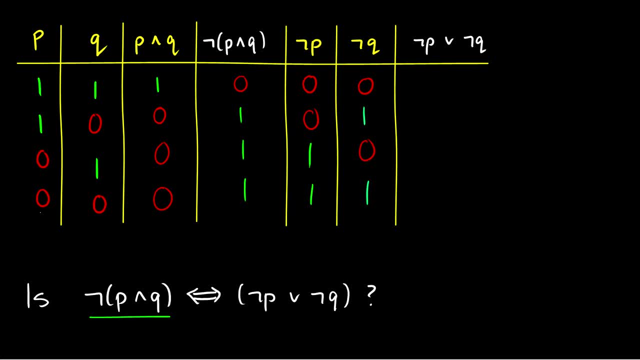 not Q is going to be true when at least one of those is true. So in the first row, not P is false, not Q is false. therefore, not P or not Q will be false. In the second row, not P is false. 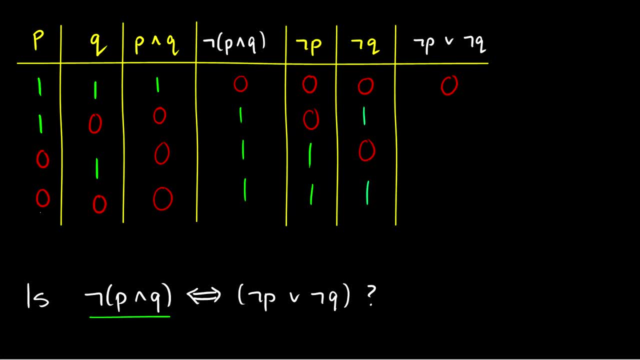 but not Q is true. so not P or not Q is true. In row three, not P is true. therefore not P or not Q is true. and in the fourth row they're both true. so of course not P or not Q will be true. 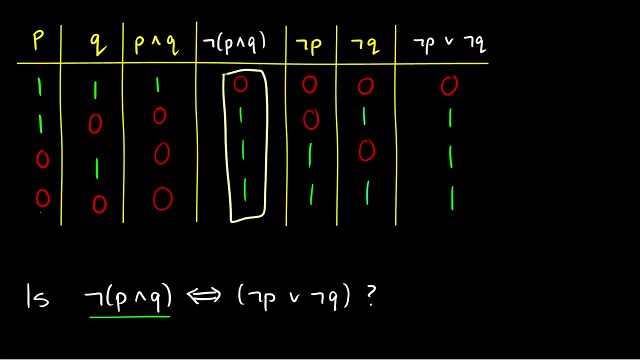 Now we can take a look at the truth conditions for the two formulas we want to compare, and they are exactly the same. Therefore, yes, they're logically equivalent, which means if I ever have not P and Q in a proof somewhere, I can substitute that in with not P or not Q, because 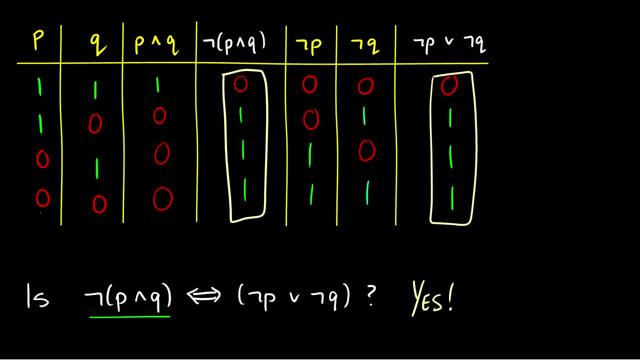 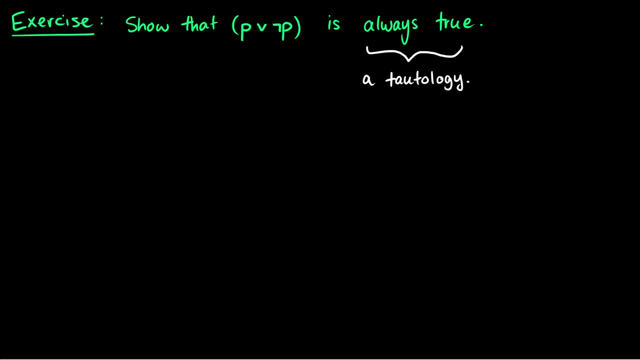 they're exactly the same thing. So that's what logical equivalence can do for us. Now I have a couple exercises. The first thing I want to do is I want to show that, P or not, P is always true- and this is known as a tautology- when it's always true. 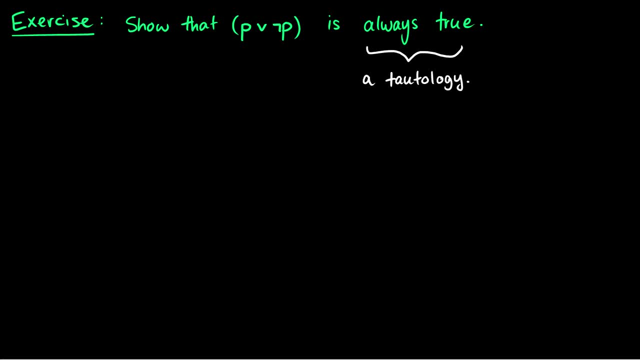 meaning that every single value in our truth table is going to be one. So let's do this, Let's build our truth table. First thing, we have to start with P, and then I'm doing P or not P. so the second thing I have to do is build, not P. 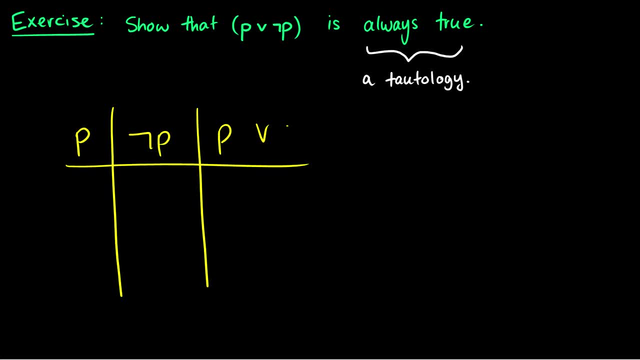 Then finally I can put them together to make P or not P. So let's build the truth table for P. Well, P can either be true or false. What does that mean for not P? Well, if P is true, then not P is false. 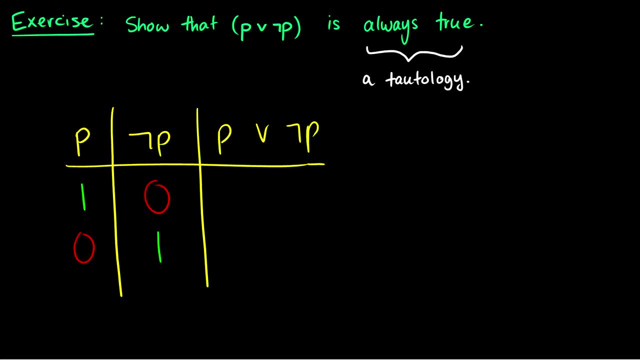 and if P is false, then not P is true. Now, P or not P is true? if at least one of them are true, Well, in the first row P is true and in the second row, not P is true. Therefore, P or not P is a tautology. 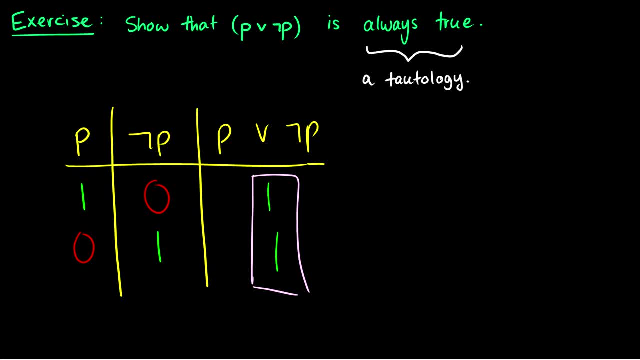 meaning that every single output is a one here. So P or not P will always be true. And, of course, P or not P could be something more elaborate, like, for instance, it might look like A and B or not A and B. So this is also P or not P. So if you treat A and B as P, then this is really just. 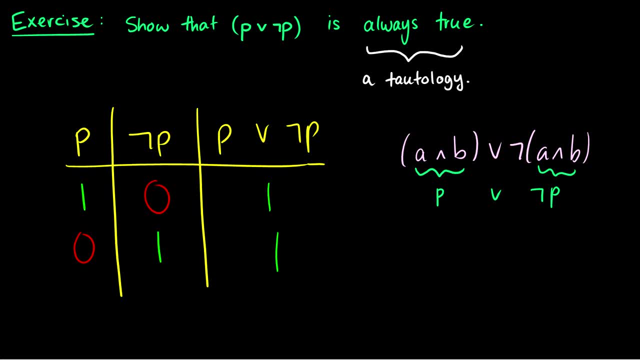 P or not P. So in a proof, these P or not P might just not be expressed with just one proposition. It might be a combination. So, just like this, A and B is similar in both, so we can treat this as P or not P, And this is another important thing to look out for. 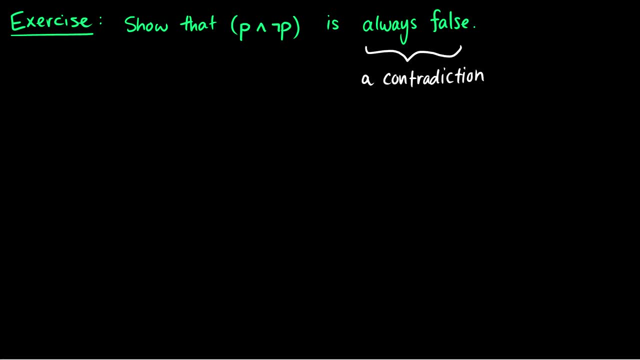 Finally, I want to show that P and not P is always false, otherwise known as a contradiction. So I can do this same thing as before, Of course. what is the truth table going to look like for p and not p, if it's? 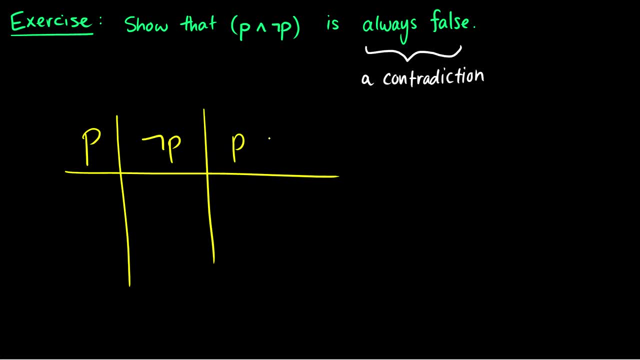 always false. Well, it means that every single thing is going to output a zero. So once again, we can build the truth table really quick. If p is true, then not p is false. If p is false, then not p is true. p and not p is true only when p is true and not p is true. but they both can't. 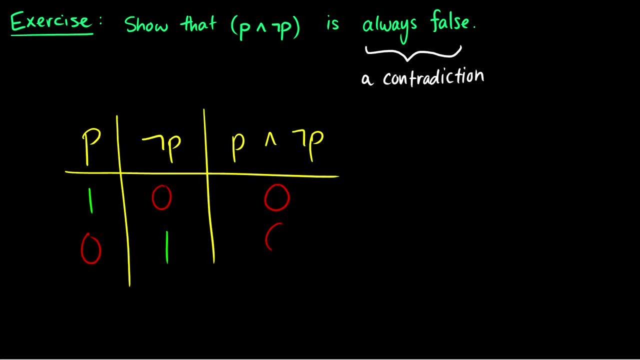 be true at the same time, So they are both false. So here, all of the outputs are a zero. Therefore, this is a contradiction. So these are proofs using truth tables. Now, this is different from proving using rules of inference, which we're going to get to eventually, and it's also